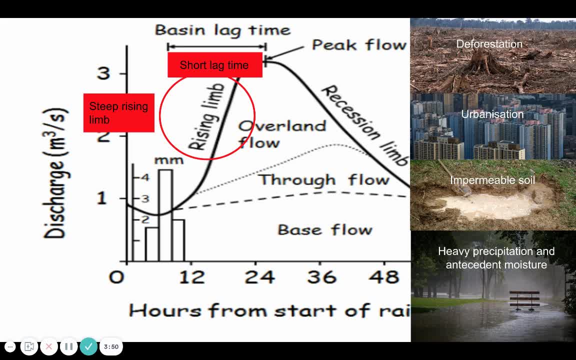 will be determined by a number of factors. right deforestation: that could reduce interception. It might mean that we have the soil- depending on what type of soil it is filling up a lot quicker, so more surface runoff and a shorter lag time. Urbanization: obviously that means that we have 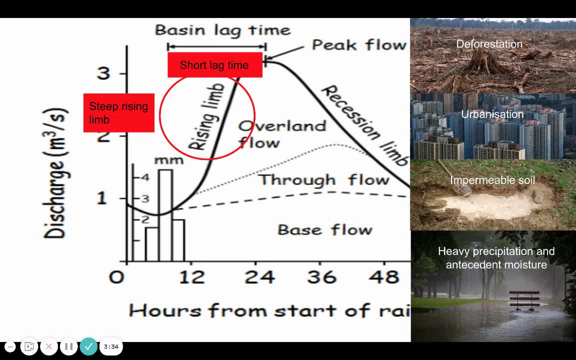 an impermeable surface right, so we've got more gutters, we've got more channels, rooftops have gutters right, so everything to get water out. So our surface is predominantly impermeable. so our main process would be overland flow or surface runoff there. 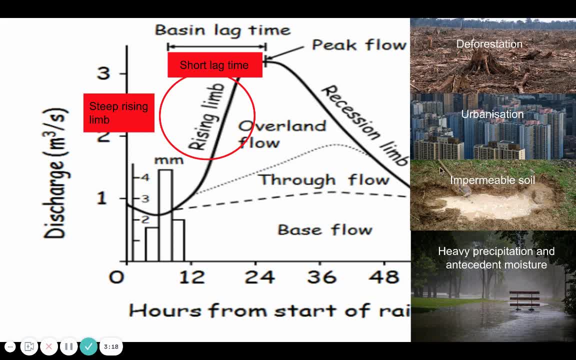 We might have soil that is impermeable, so very clay-type compact soils. So I might look at the geology, right. so the rock type, the surface type and the precipitation, both type and intensity as well, all right, and also the antecedent moisture. so how much moisture is already in the soil if? 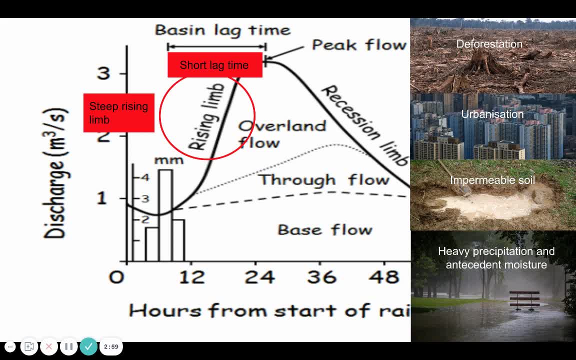 there is soil as well. There are other things that I could take into account that could be relief. if it is a very steep gradient, then obviously there won't be time for infiltration, so I might have a very short lag time here as well. all right, So if you're asked to sketch one of these, 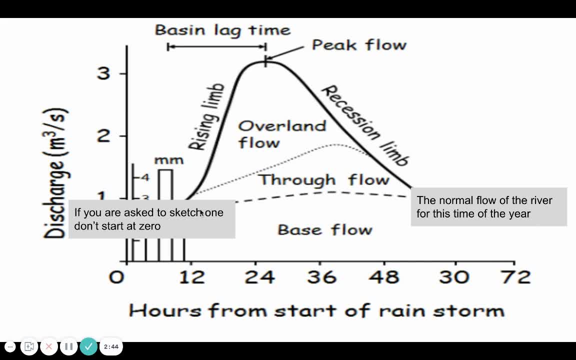 remember, don't start at zero, because you're showing me that there would be no water in the river channel. Base flow here shows the normal flow of the river for this time of the year, so if I have seasons, then base flow varies. right Now this is something that is completely 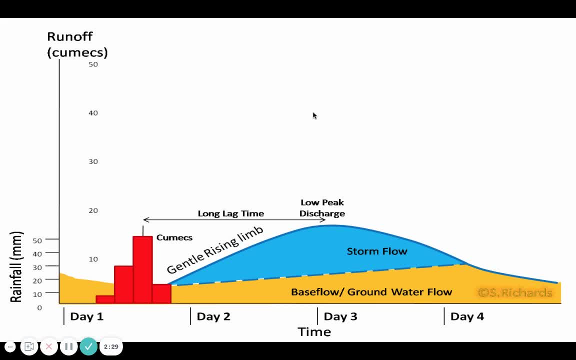 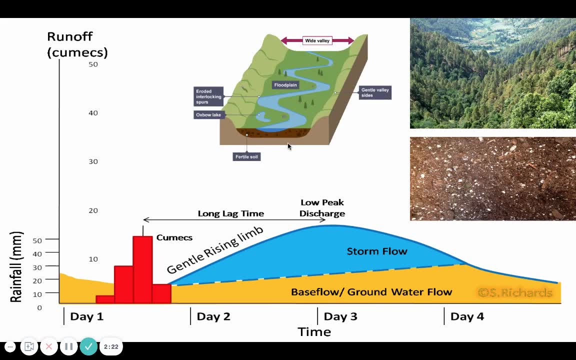 different. I can see here I've got a flood hydrograph with a long lag time and a low peak discharge right, so I'm going to have predominantly a lot of through flow. that would be my main process right Now. I could have lots of vegetation. if I'm having a long lag time, my surface soil 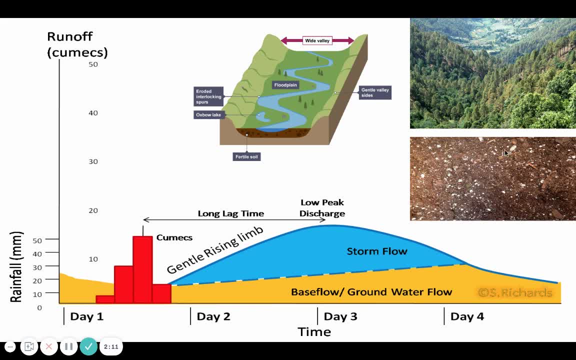 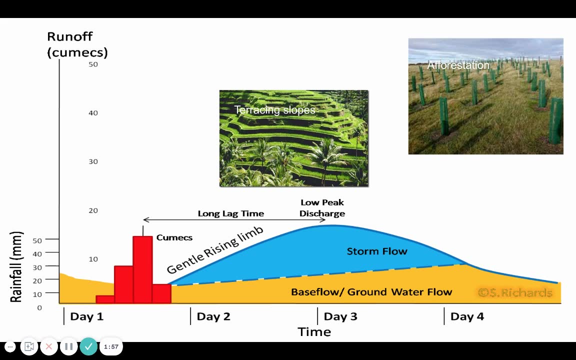 might be made up of porous or sandy type soil which allows a lot of infiltration. It might be very, very flat, so a floodplain area which also allows a lot of infiltration as well here, Okay, things I can do to manage my lag time. obviously I want my lag time to be a lot longer. 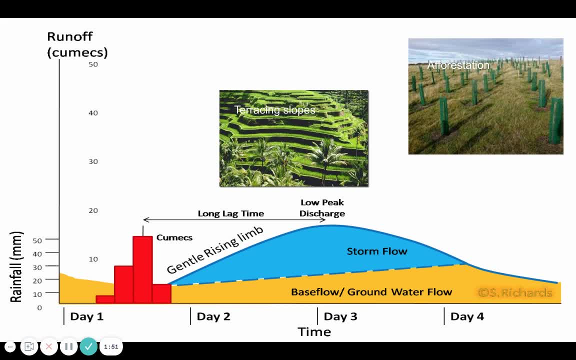 that means I'll have lower peak discharge and more through flow being the dominant process, as opposed to surface runoff. I could terrace slopes, right, You can see these terraces here. that would give time for infiltration to occur. I could plant trees, obviously.